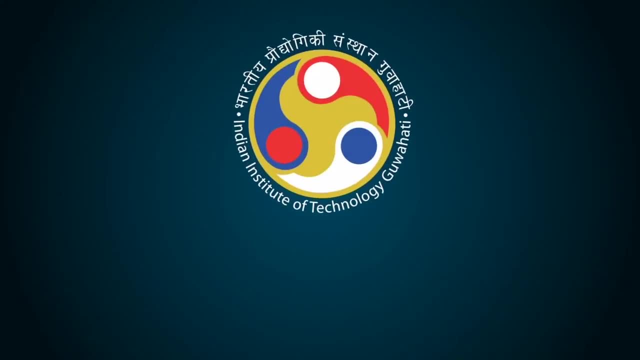 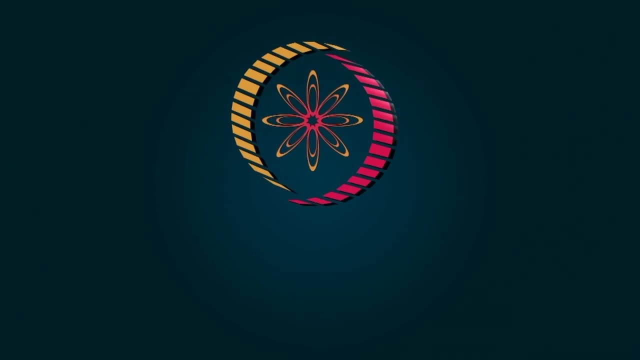 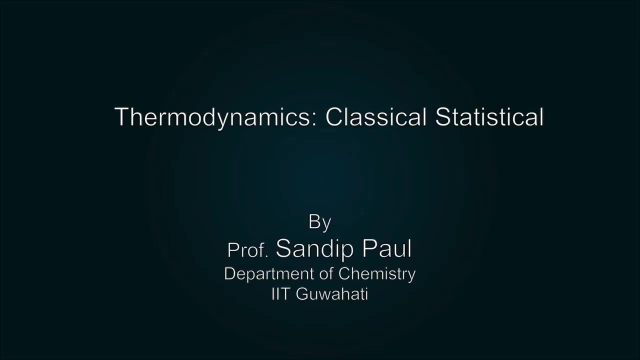 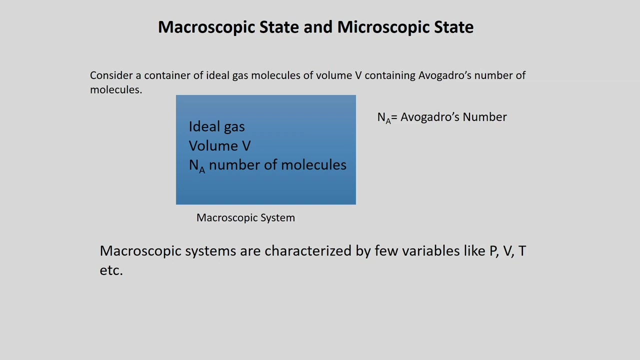 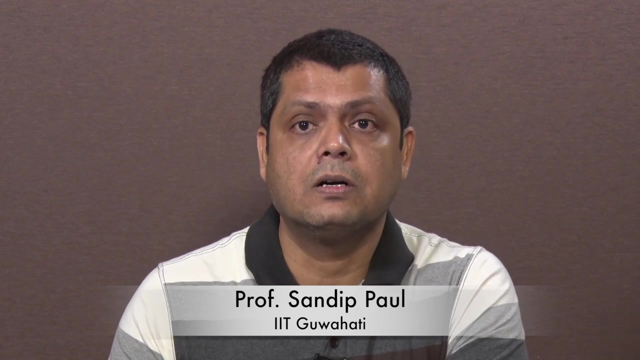 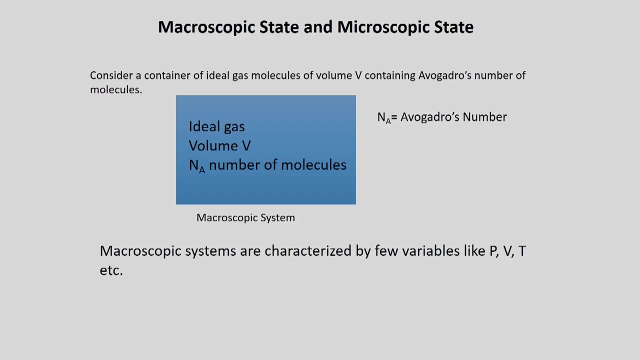 Thank you for watching. Okay, so today we will discuss macroscopic state and microscopic state. For that, we first consider a container of ideal gas molecules of volume V containing. this container contains Avogadro number of molecules. Okay, so this is the container. this is the container, Okay. 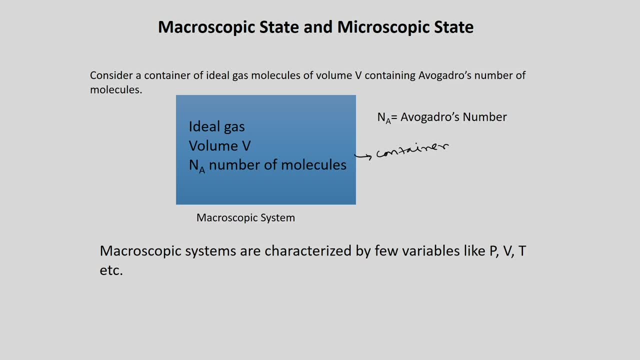 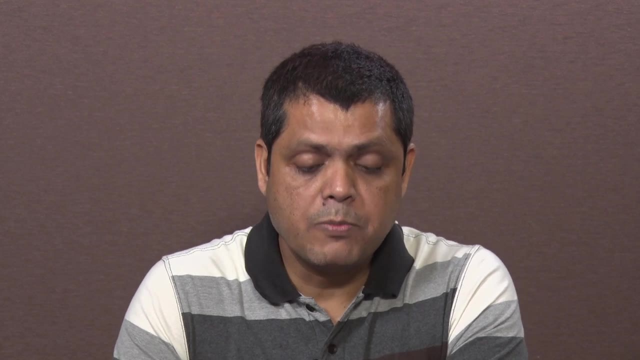 so we consider one container contains ideal gas and the volume of the container is V and in that container we have kept Avogadro number of molecules. So this is a description of macroscopic system. Okay, so macroscopic systems are characterized by few variables like pressure. 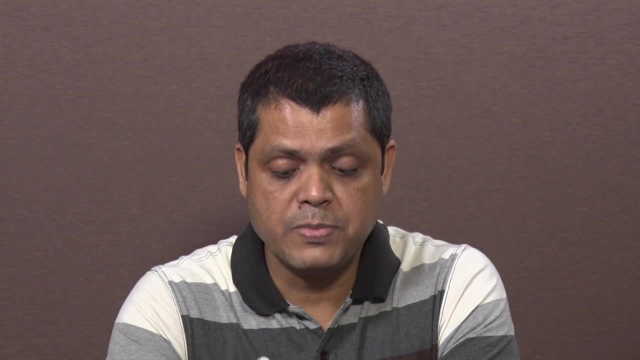 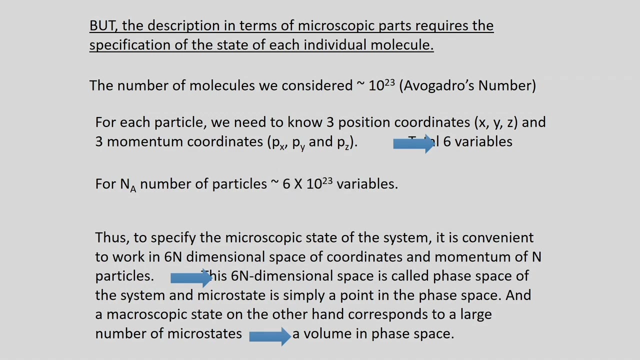 volume, temperature, etc. So we can observe what is the pressure here or what is the temperature here, etc. Okay, but the description in terms of microscopic parts requires the specification of the state of each and individual particle. So while we discuss about macrostate, there we did. 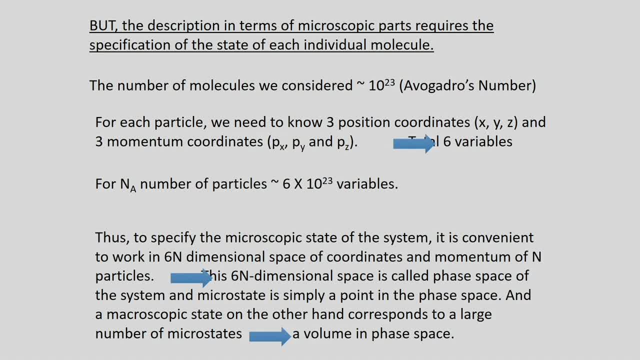 not consider the how, the what is the contribution to the pressure of each and every particle? okay here, But description, if you in terms of microscopic part, requires the specification of the state of each and individual particle. Okay, Okay, Okay, Okay, Okay. 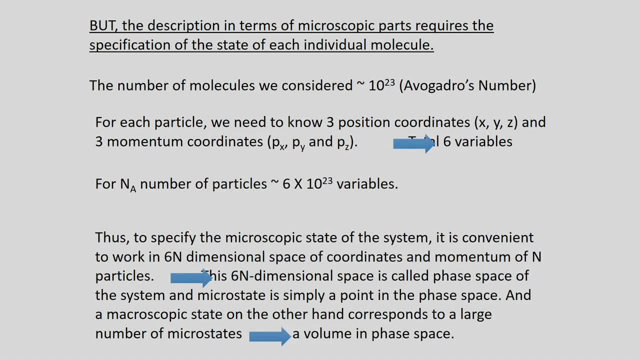 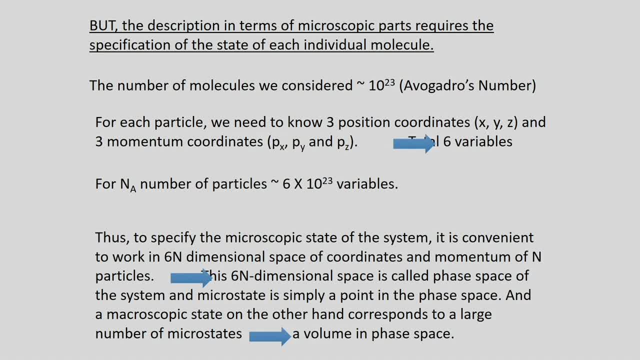 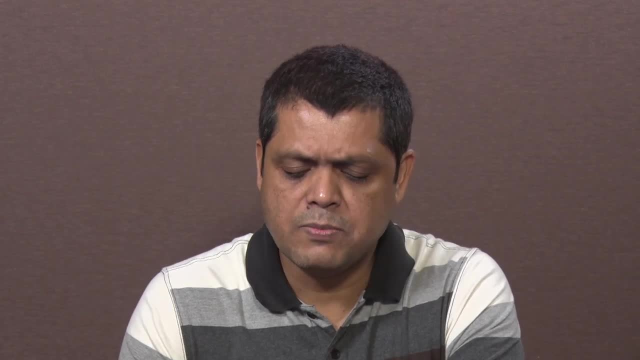 coordinates. Okay, So total 6 variables. we need to know for each particle- And we have used Avogadro- number of particles here, so typically we need 6 times 10 to the 23 variables. Okay, Thus, to specify the microscopic state of the system, it is convenient to work on 6. 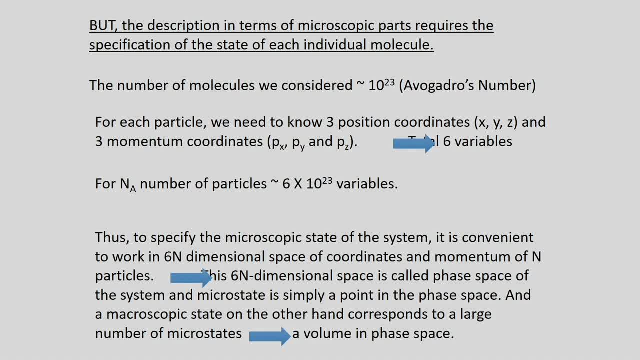 n dimensional space of coordinates and momentum of n particles. This 6 n dimensional space is called phase space of the system, And microstate is simply a point in the phase space and the macroscopic state, on the other hand, corresponds to a large number of microstates and it represents. 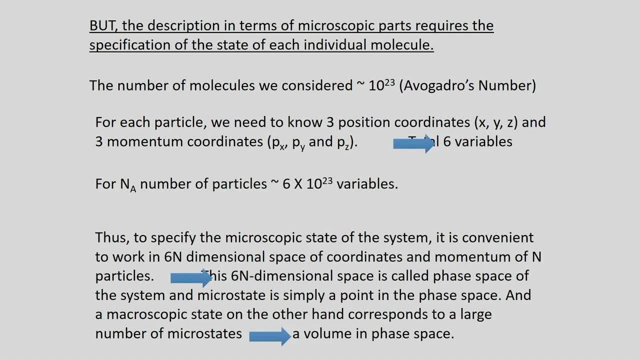 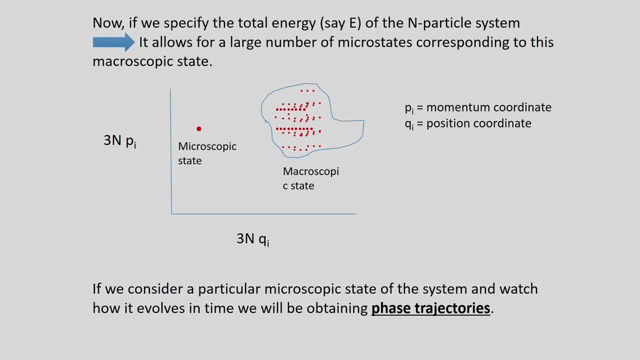 a volume in the phase space. So we can see it in this plot here. Now, if we specify the total energy- suppose total energy say E- of the n particle system- it allows for a large number of microstates corresponding to this macrostate. So as we see that we have a 6, 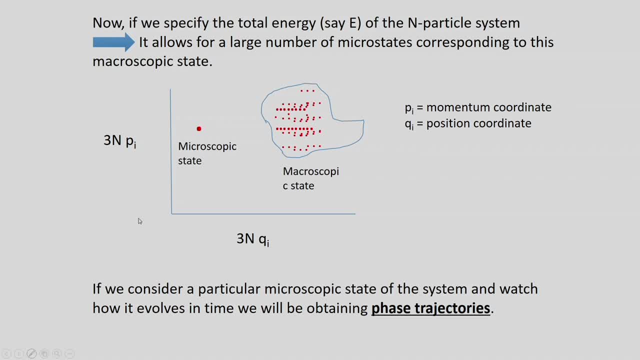 n dimensional space space here. So here we plotted 3N number of momentum coordinates versus 3N number of position coordinates. and macroscopic state is only a point in that phase space. On the other hand, the macroscopic state, it is a volume in the phase space. 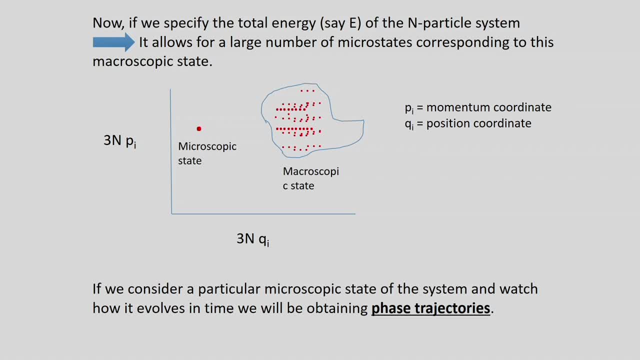 So if you consider a particular, consider particular microscopic state of the system and watch how it evolves in time, we will be obtaining phase trajectories. So what is phase phase trajectory? So if you consider a particular microscopic state of the system and watch how it evolves in time, we will be obtaining phase trajectories. Now we will. 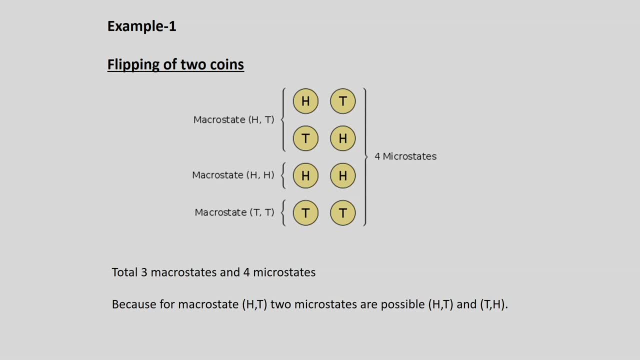 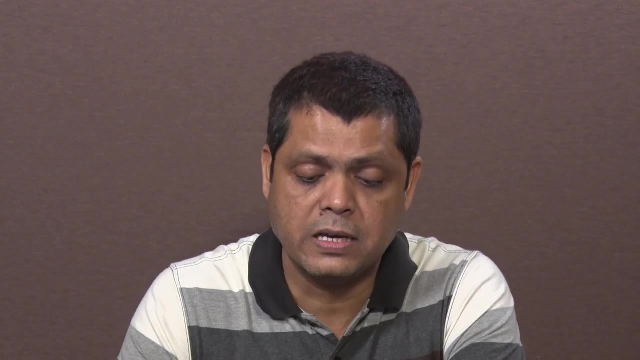 hear today here. consider two examples for better understanding of microstate and microstates. Suppose we are flipping two coins. So one possibility is first coin comes with head and second coin comes with tails. So this is the first occurrence here. Then next occurrence. 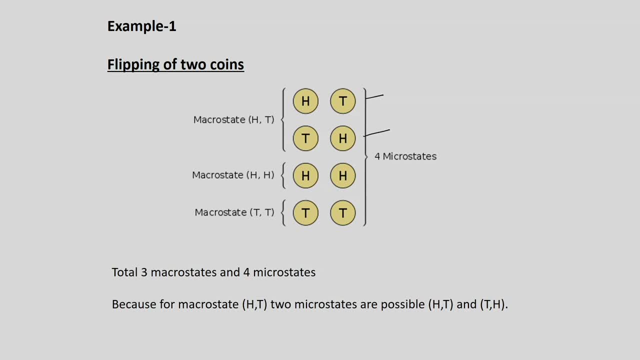 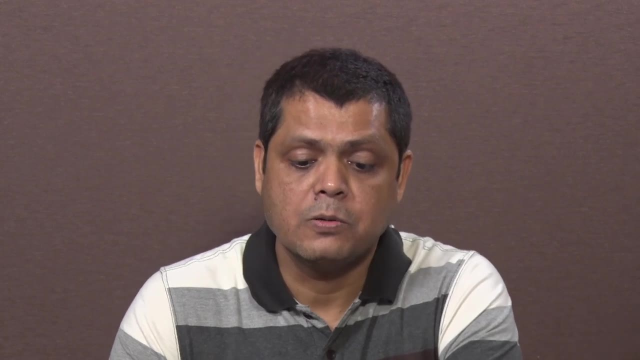 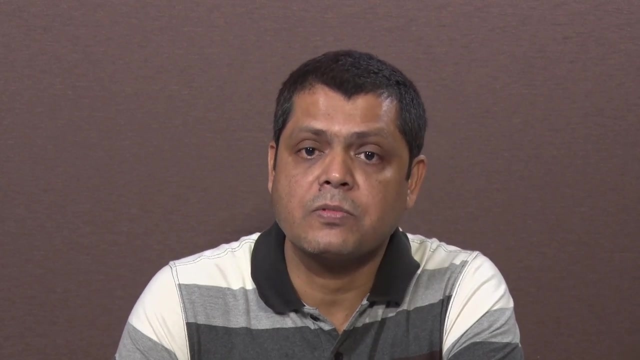 is first for first coins. first coin we get tails, and for the next second coin we get heads. So for this microstate means one head and one tail. we have two microstates: First we have head, then tails or tails heads, like this. Similarly for microstate H, H means for. 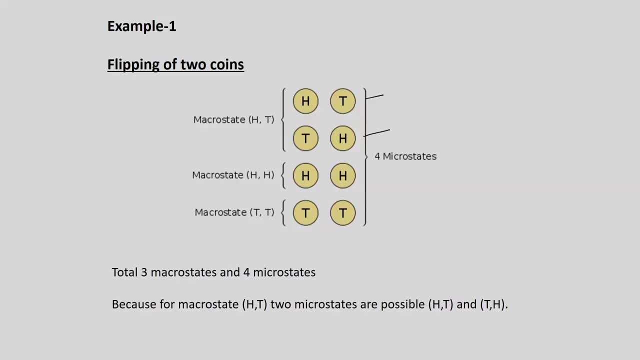 both coins if we get heads. So for this macrostate we have only one microstate. So for this one, for H, T or T H, we get two microstates. For this one we get one microstate. H H case, and we can also. 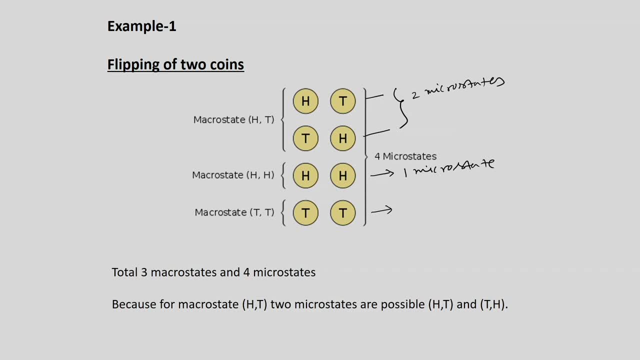 get tails, tails, both the coins for both the coins. So for this one we get, for this, macrostates. we macrostate will be defined by T, T. here we get one microstate. So we have total three macrostates. What are those macrostates? One head, one tail. 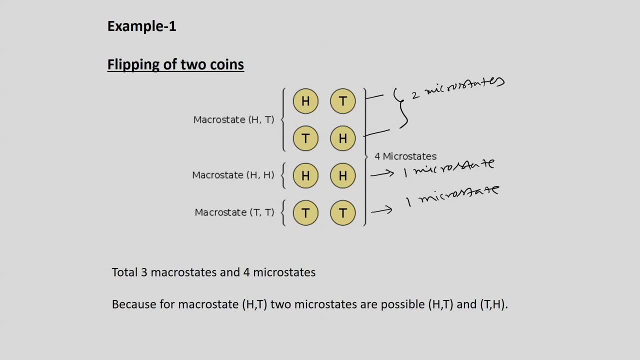 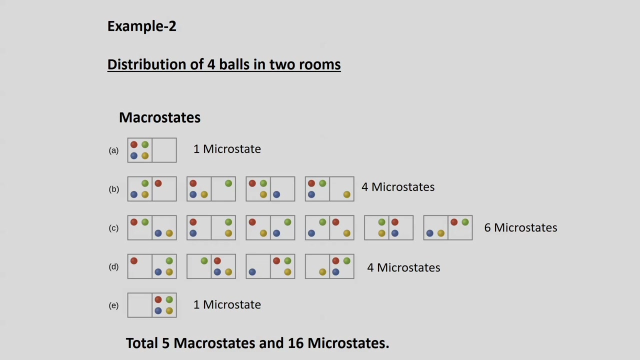 is one macrostate, both the heads is one macrostate and both the tails is the third macrostate. And how many microstates we have? We have four microstates, because macrostate H, T, head, tail contain two microstates like H, T or and T H. Next we take another example. So we have, suppose, four walls and then we 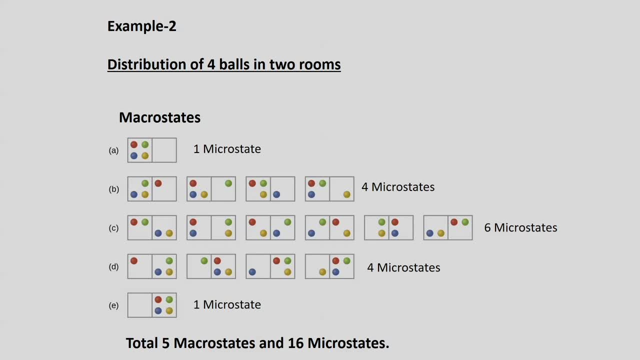 have two rooms or two baskets, whatever you say, And these balls, they are identified by different colors. Now, if, Now if I ask you, you put four balls in different manner, what are the possibilities? One first possibility is: all four balls are in the first room and there is no ball in the second room. 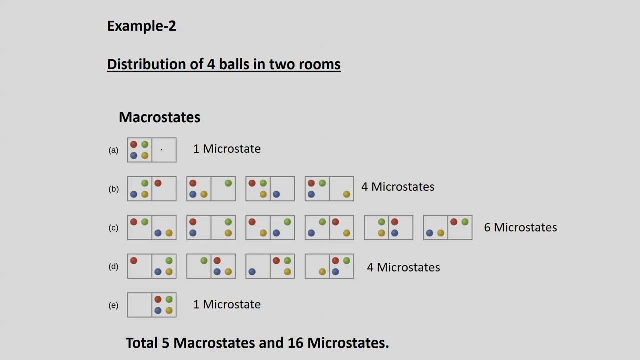 So this is one macrostate possible. So this is microstate. one microstate like this: Then we can have blue, red and green ball in one room and a red ball in second room, And now we can change the ball means three balls in one room. 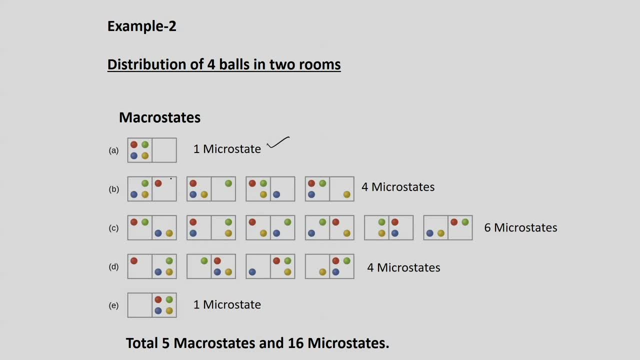 three ball in first room rather and one ball in second room. Okay, So for this kind of arrangement we get four microstates. Now we can have both rooms. we can have equal number of balls means two, two. Okay. Now if we rearrange new virtual ball, we could 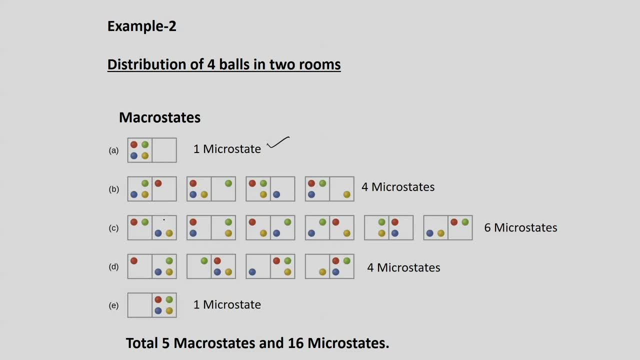 also change. golden ball, which is green, we can have. golden ball is blue and green balls can be any. Now, because we have keywords here in the second column. however, if ourOWsiscilla underscore, its is in the quarter column where we rearrange the balls. so we get six different possibilities here And then in the fourth. 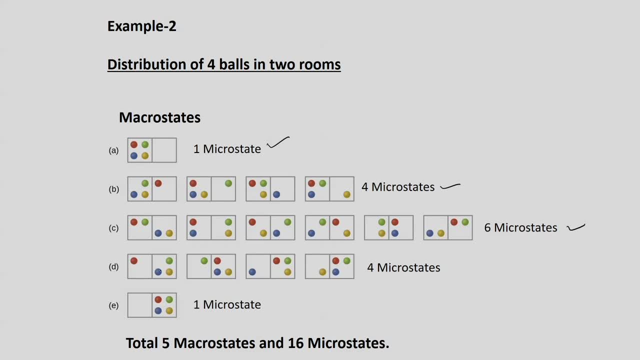 case. suppose we put one ball in first room and three balls in the second room, And for this case we get four different possibilities. And the last case: the first room is empty and the second room contains all the four balls. So how many macrostates we have now? 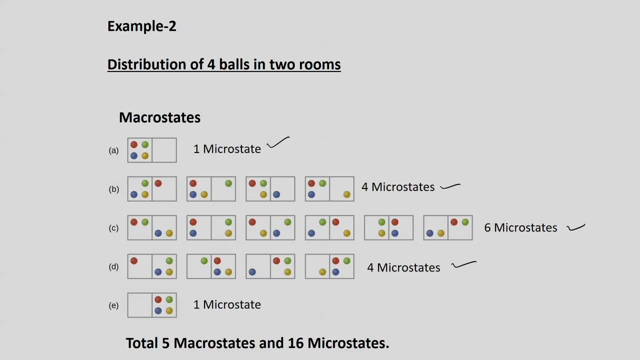 We have five macrostates. And how many microstates are there? We have 16 microstates. Like for the first macrostate, we have only one microstate. For the second macrostate, we have four microstates. For third microstate, we have six microstates. For fourth macrostate, we have four microstates. 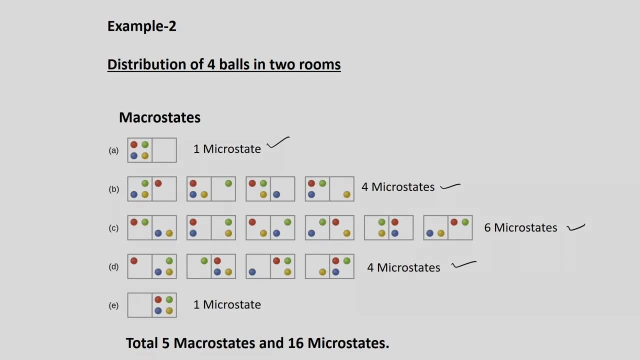 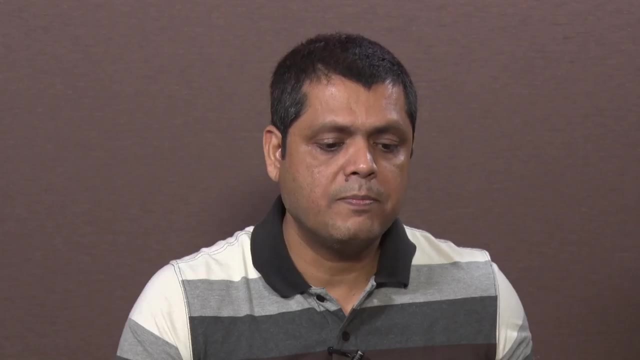 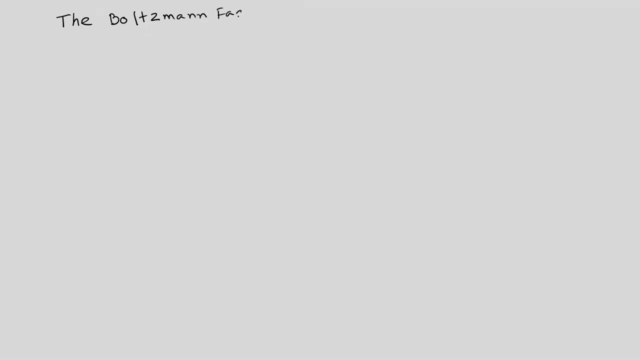 And for fifth macrostate, we have only one microstate. Okay, So now we understand what is macrostate, what is microstate? Next we start with Boltzmann factor. So now we discuss Boltzmann factors. Okay, All of you know Schrodinger equation. 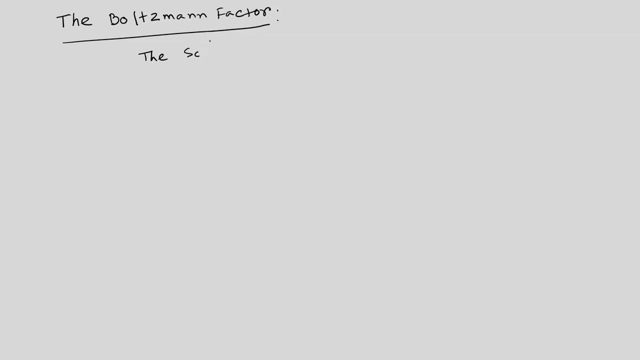 So you know, when I talk about Boltzmann variable, you think that for n bodies, for n existing Squeezie, Okay, And you know, earlier on you talked about that, the' Like: if you are своих, Alright. 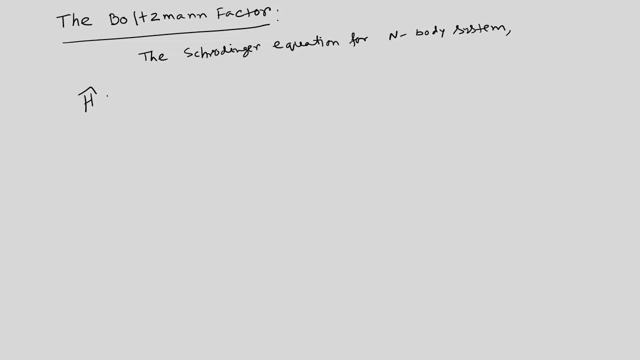 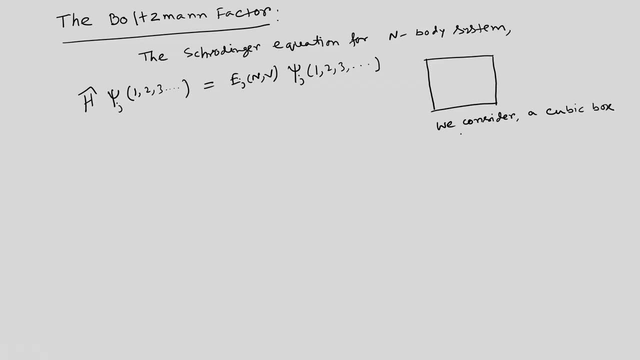 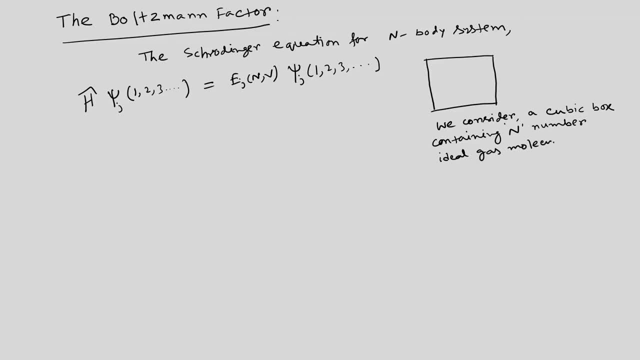 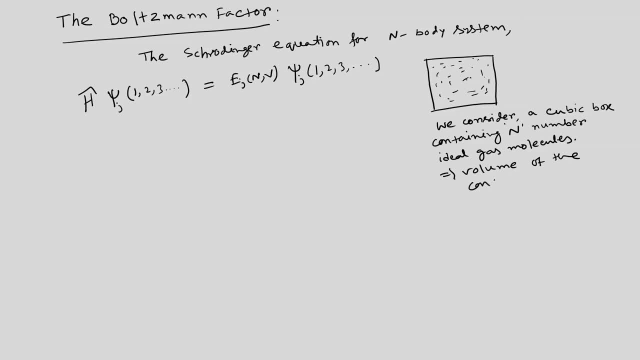 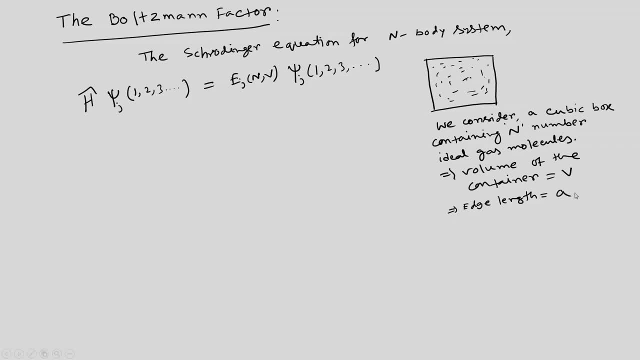 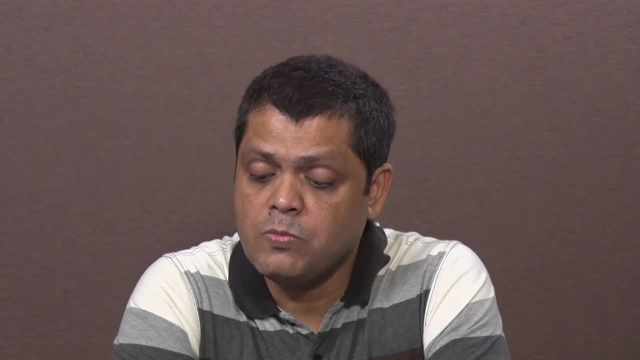 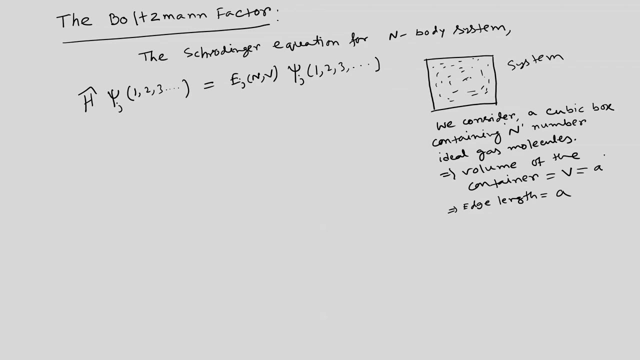 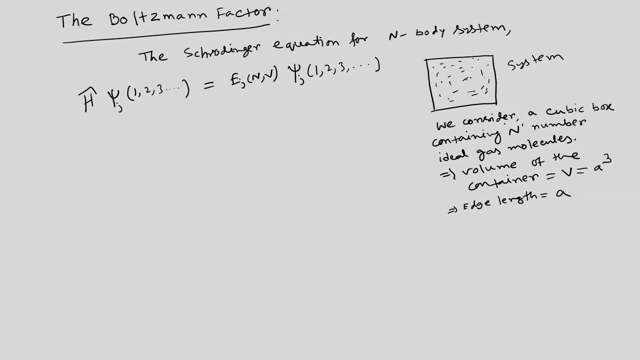 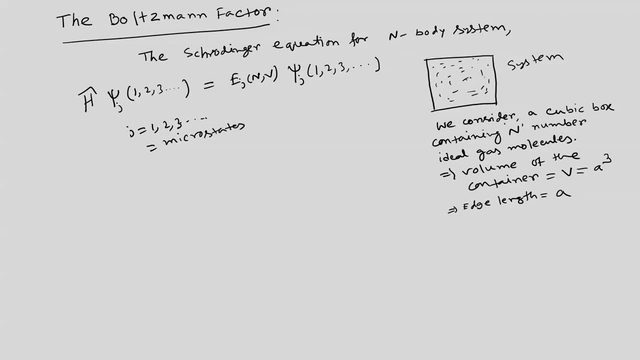 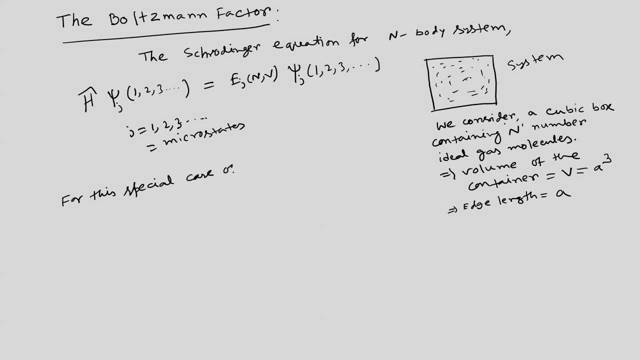 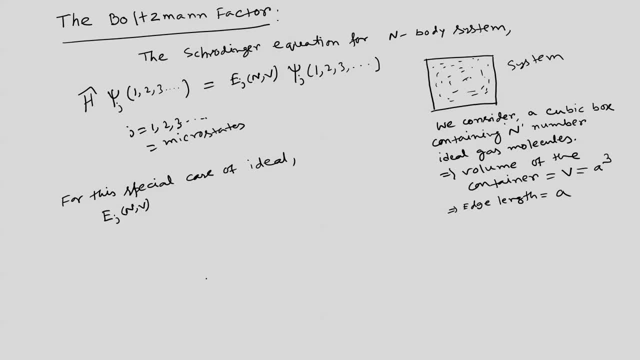 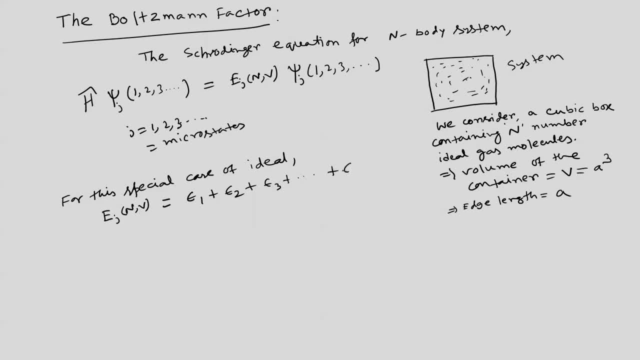 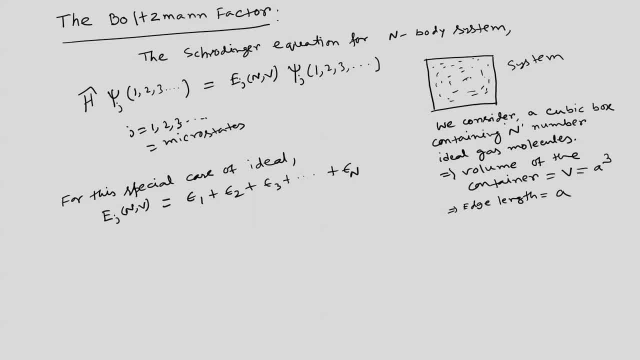 E j. So we considered: of particle 1, coordinate of particle 2, coordinate of particle 3, etc. Now, so E j is like this: So if we say the E psi j equals to E j psi j, this is our equation 1 and we can say: this is: 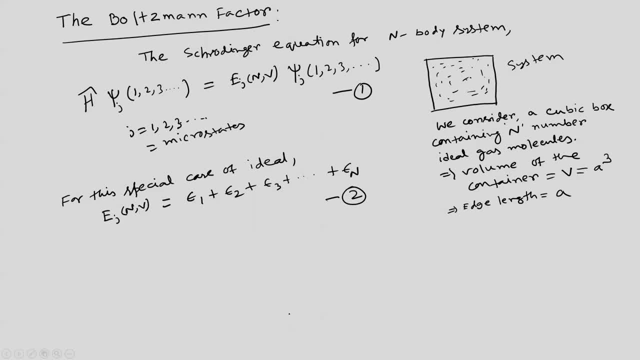 our equation 2.. What are those? epsilon 1, epsilon 2, etc. So epsilon 1, epsilon 2, etc. are the individual molecular energy. okay, So in the expression of E j means E j equals to epsilon 1 plus epsilon 2, this expression 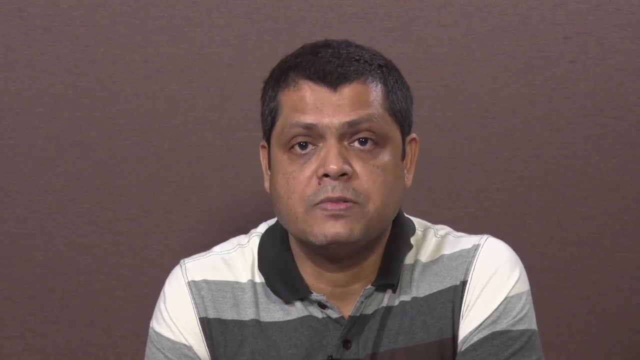 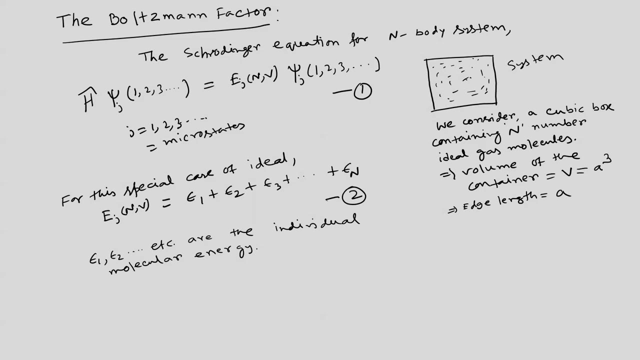 2. It contains E j In number of terms. number of particles. it depends on number of particles, So E j depends on number of particles. okay, So that is how the independency of E j comes here. okay, And we can add them the molecular energy levels, because epsilon 1 plus epsilon 2, etc. because 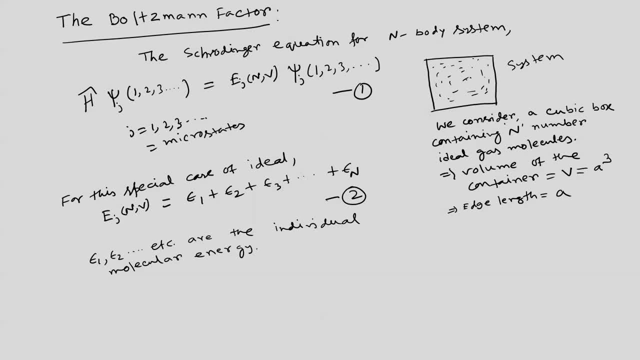 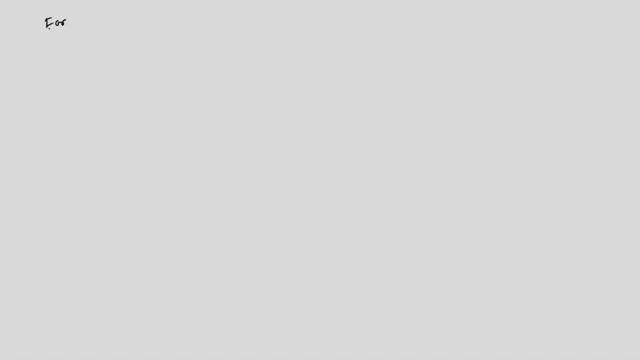 we are considering here ideal gas, For example, for a monoatomic ideal gas. okay, if we consider a monoatomic ideal gas in that container, okay, Okay, Okay, Okay, So in the container, this presented above, presented here, or consider here, consider. 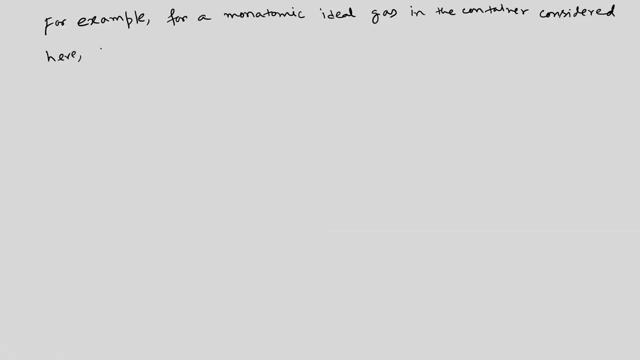 here If we ignore this. Okay, Okay, Okay. So let us consider the electronic states and focus on the electronic states and focus only on the translational states. then E? j's, epsilon j's are equal to epsilon 1 plus epsilon 2.. 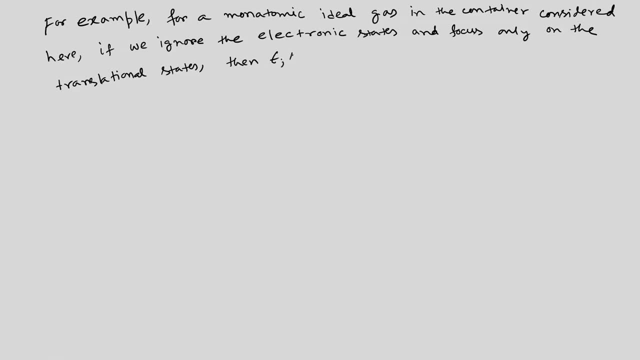 Okay, Okay, Okay, Okay, Okay, Okay. So epsilon 1 plus epsilon 2 are just the translational energy given by. so we consider three dimensional box. epsilon nx, ny, z is h to the 2 by 8, m a to the 2, like this, since we consider a three, 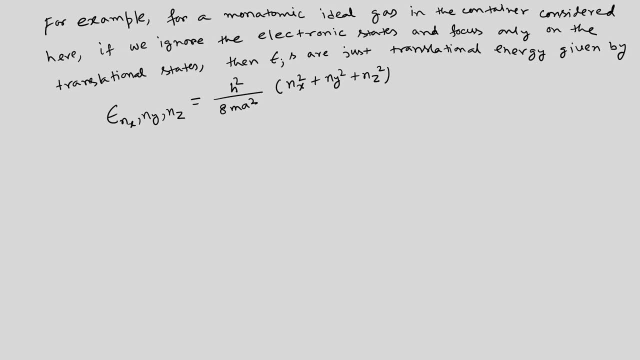 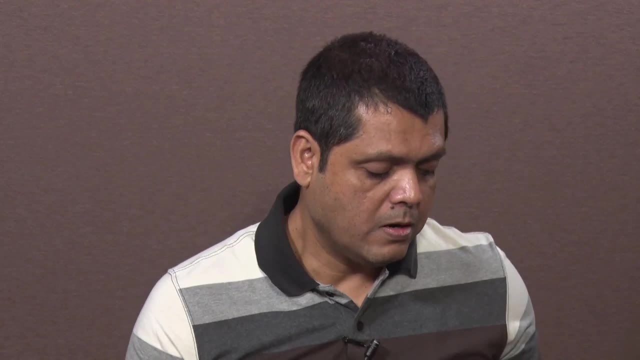 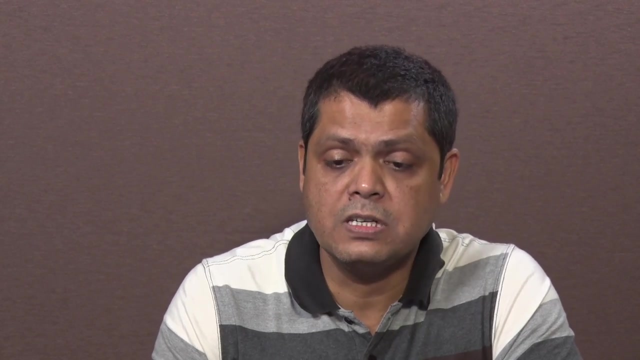 dimensional box. we get this expression, So this is related to, you know, the particle in one dimensional box. so this is for energy value, for energy expression, for particle in three dimensional box. Now, how does the V dependency comes? we discussed, how does n dependency of ej nv comes Now? 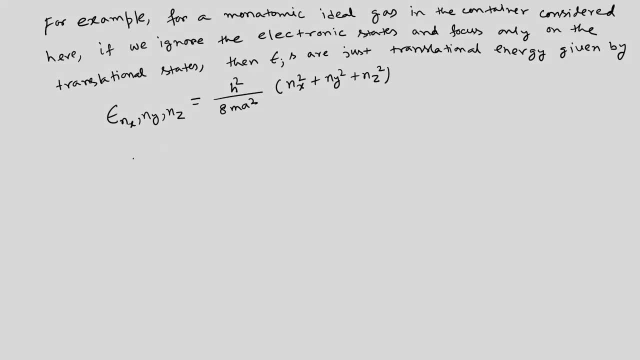 the V dependency comes. so if we see this expression here, we see that there is one term called a to the 2.. So in the above expression We have a term a to the 2 in the denominator right, okay, and we know, and a is nothing but. 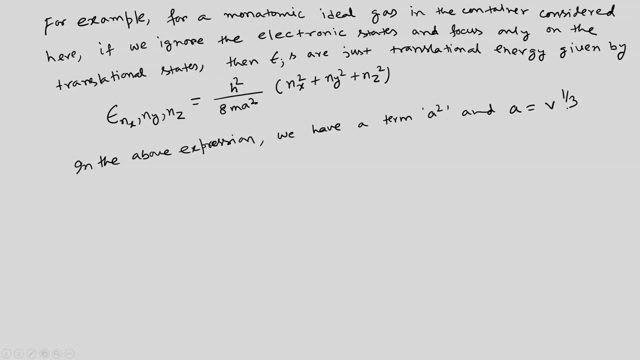 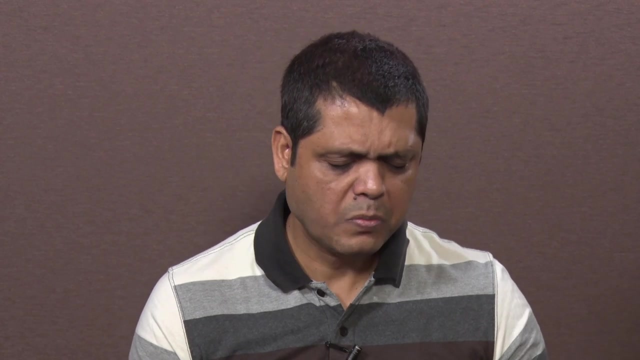 V to the one-third right. we consider cubic box. Okay, Okay, So it says so. or it depicts the volume: dependency V, dependency V, dependency of ej. So now we know. how does ej come? Okay, Okay, So ej depends on n and depends on V. okay, So what? what is our goal? okay, So, our goal. 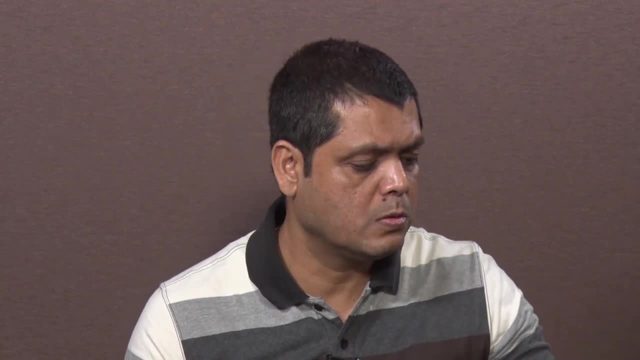 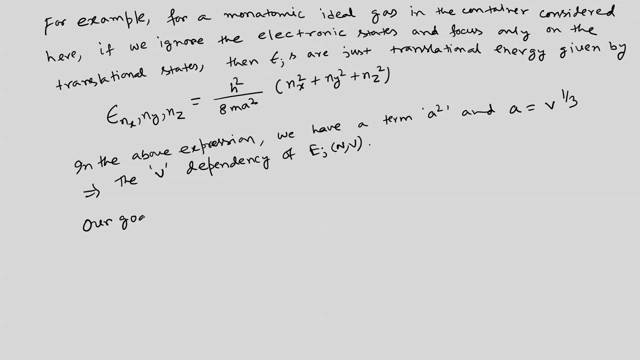 is to. our goal is to okay, our goal is to know our goal. So what is our goal? So we want to know, Okay, Okay. So we want to know the probability, the probability that a given or that a system will be in the 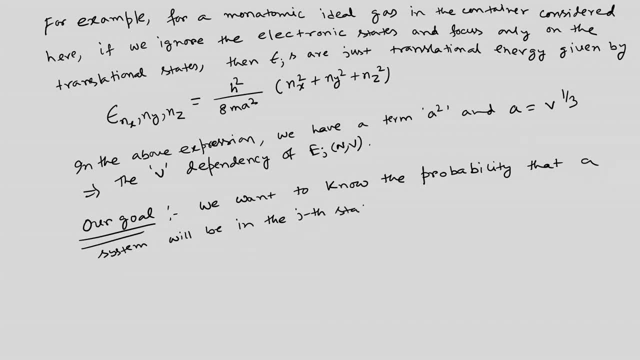 zth state: Okay, Okay, I mean energy, Okay, Okay. So having energy Okay, Okay With energy, Okay With energy, Okay. So we want to know the probability, because if we know the probability then we can calculate. 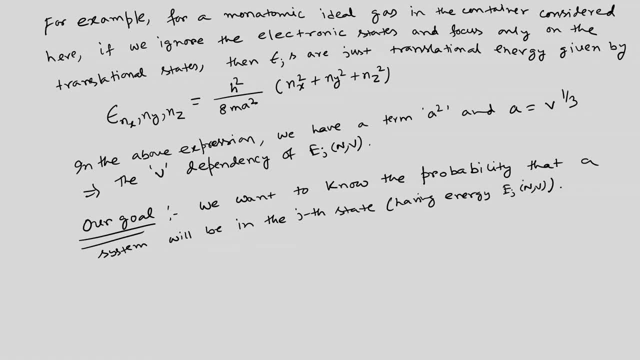 the average quantity, right with the help, Okay, that we discussed in the last class. So to do this, for this we consider a huge collection of systems in contact with the heat reservoir. at temperature T, Each system has the same values of a number of particles, volume and temperature. 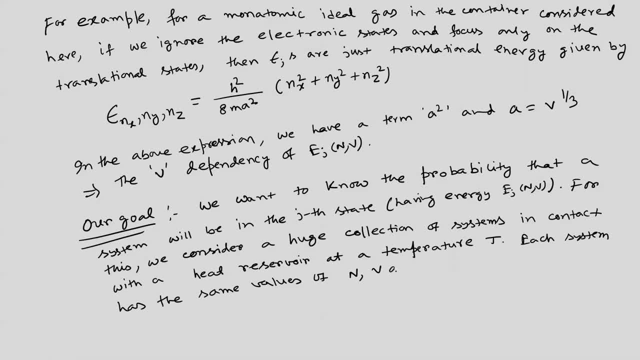 Okay, But but is likely to be to be in different quantum state. quantum state consistent with temperature, T. Okay. with the values of a, n and v: Okay, such a collection of systems is calledsay values of a, n and v. Okay, 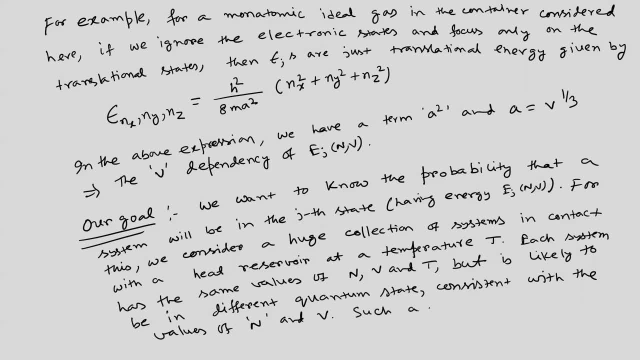 Okay, Such a collection of systems is called a collection ofsted хочет this, so it will be one known concept. Okay, That means such a special collection will be there and it can be used for decades, right? That is why such a collection ofv-it is also called the collection of네요htrہt eise. 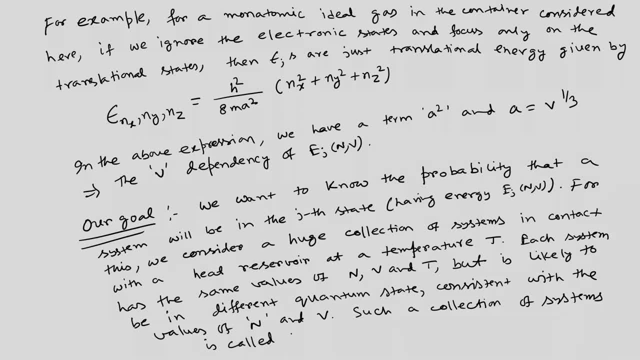 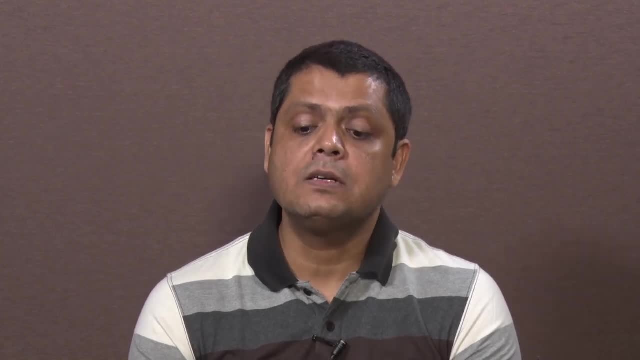 an티 eise naying tree. So for this, actually, what is our goal? Our goal is to know the probability that a system will be in the jth state, having energy E, j. For this, what we consider, We consider a: 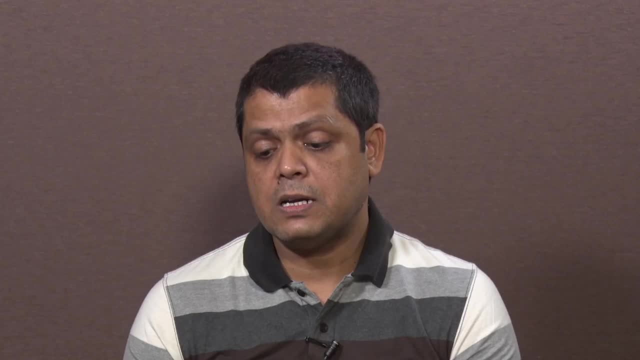 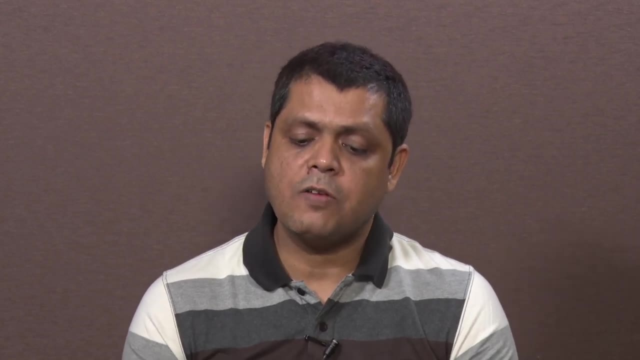 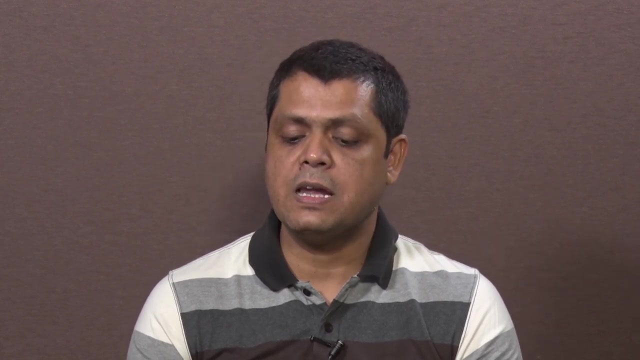 huge collection of systems in contact with a heat reservoir at a temperature T. The system in that collection has the same values of n, v and t, but is less likely to be in different quantum states consisting of the values of n and v. Such a collection of systems is: 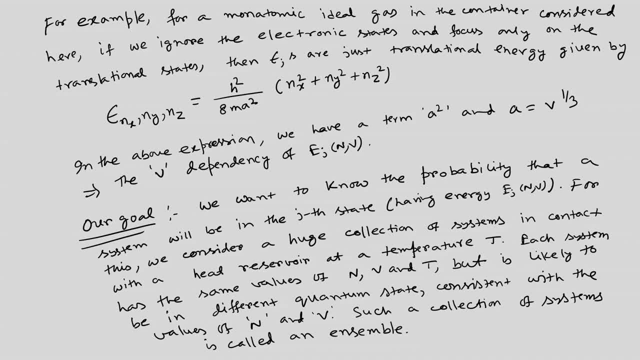 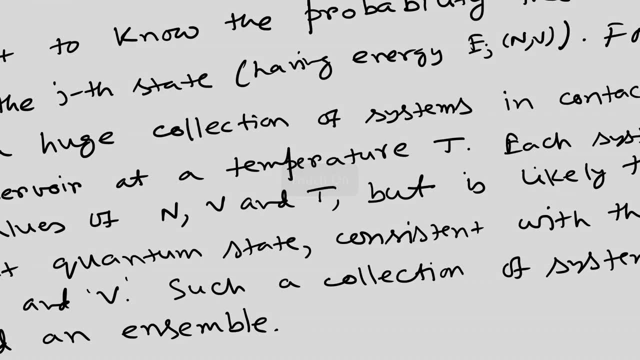 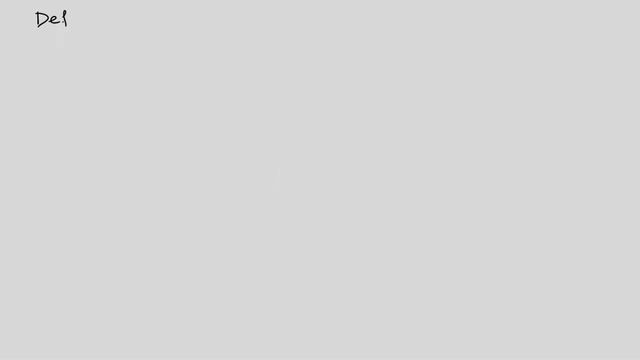 called an ensemble. What is the definition of the ensemble? Next, we will just define it. Höf�� Regression N- singles is the definition of actual definition of Enzimbel. So it is an idealization consisting of consisting of a large number of mental copies, sometimes. 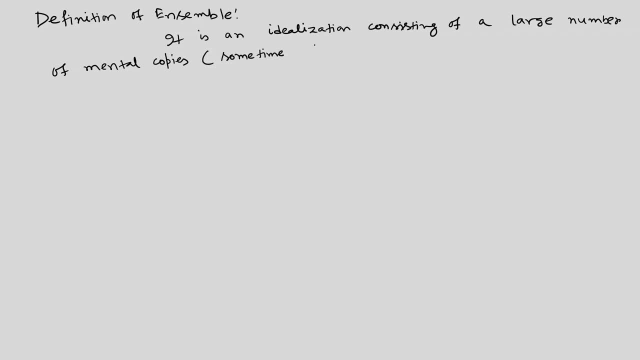 And considering a infinitely many, So we considered many, many or a huge or large number of mental copies of a system represents a possible state that the real system 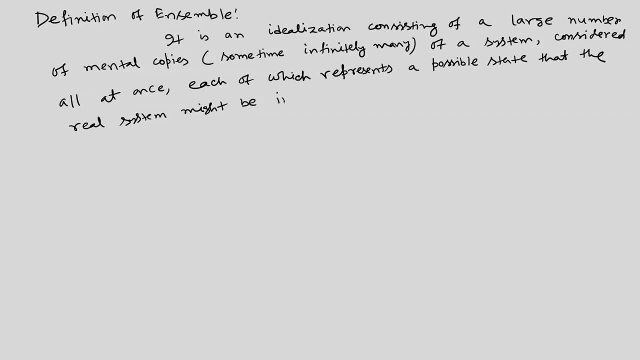 might be in. So what is the definition of ensemble? Ensemble is an idealization consisting of a large number of mental copies- sometimes infinitely many- of a system considered all at once, each of which represents a possible state that the real system might be in. So 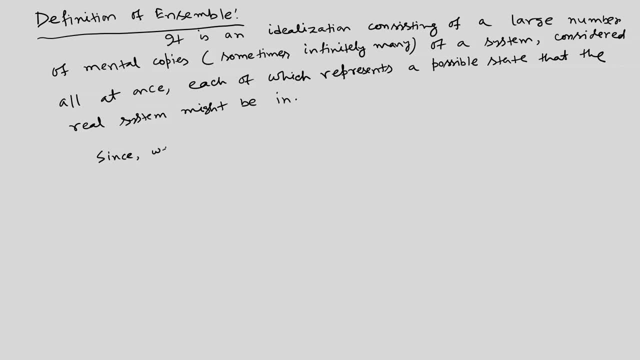 since we consider constant in V, t. So we are basically describing canonical ensemble, canonical ensemble, So in canonical ensemble. number of So in canonical ensemble. number of So in canonical ensemble. number of particles, volume of the system and temperature are fixed. 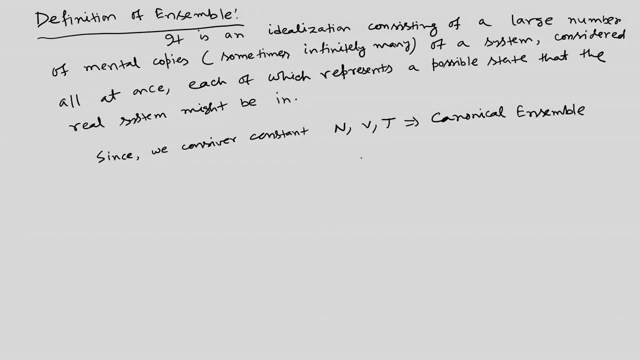 So now, basically, what is the ensemble? If we represent pictorially, we get like this: so on study. So these are the mental copies of our system and they all are having constant n, v, t and the whole thing. ok, So let me draw it again little bit better. 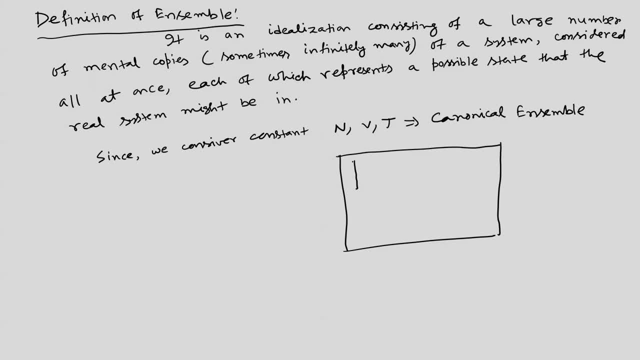 manner. So we have like this: ok, So all are having in same number of particles, volume and temperature fixed, etc. ok, So we have heat reservoir here and whole thing. if we just putting one insulator here, So isolated from whole thing, whole thing is isolated. 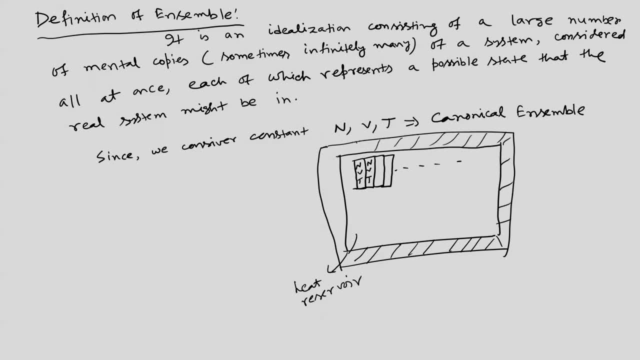 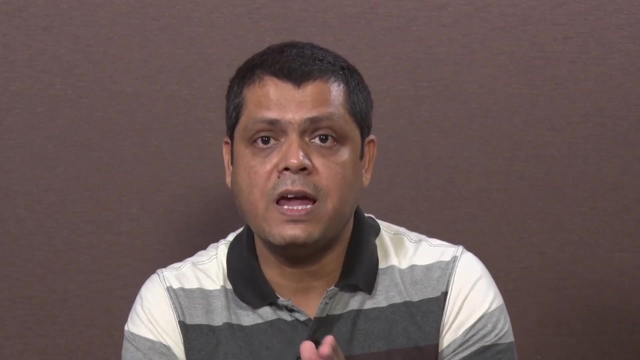 from the surroundings. ok, So we have insulator, thermal insulator. So these are all mental copies. ok, So our goal is to find a state J having energy, E j, and for that what is the probability? ok, That is our goal. ok. 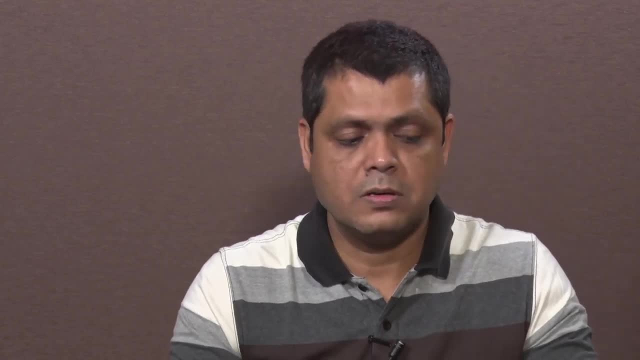 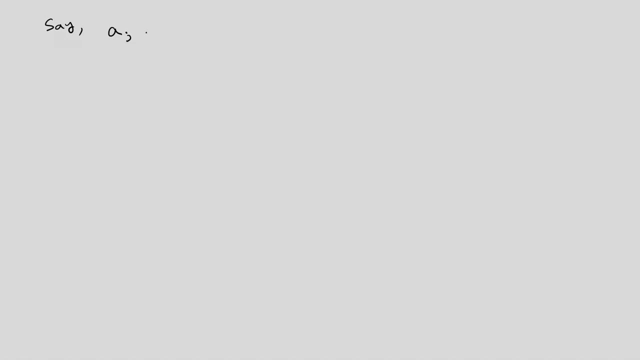 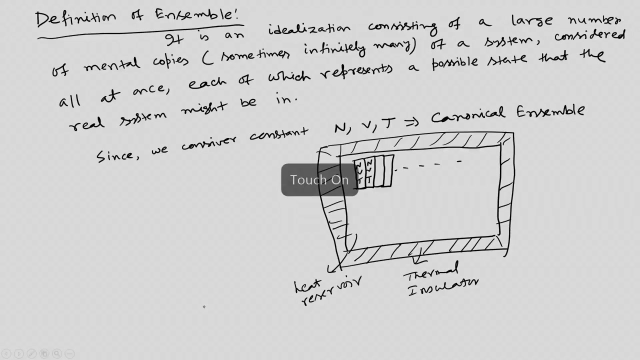 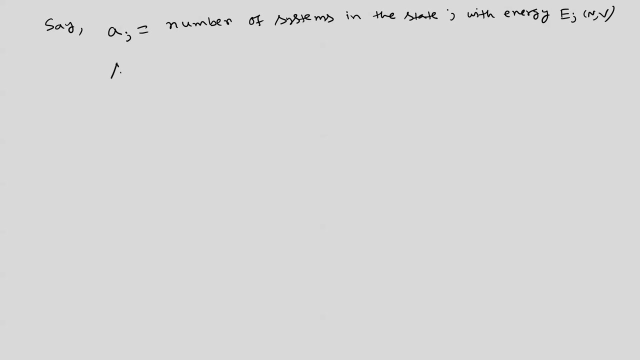 So we define, say A j, defining one quantity: A j is number of systems in the state J, with A j. So we are, our goal is to calculate, ok. So how many systems are there in the J state having energy? E j that we called A j, ok, And capital A represents total number of systems. 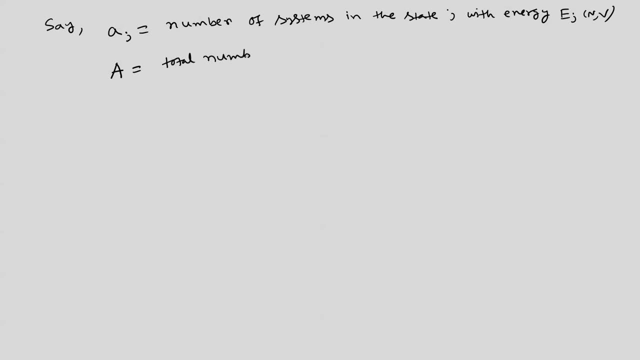 And this A is very large, usually very, very large, very large number we consider ok. So we defined two quantities: A, j and A j. A: j is the number of systems in the state, J with energy, E? j and capital. A is the total. 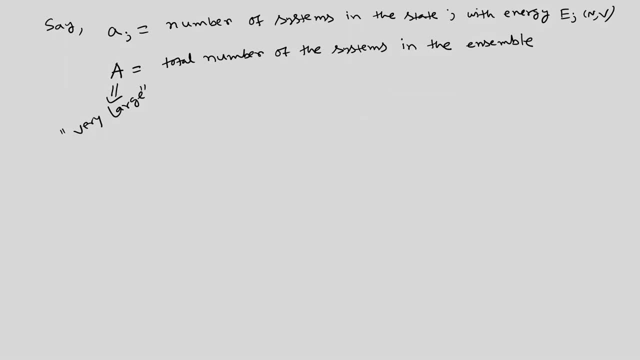 number of the systems in the total number of the systems in the ensemble. ok, ok, So now we the relative number of systems In the states with energy- E 1 and E 2- must depend on the number of systems in the state. 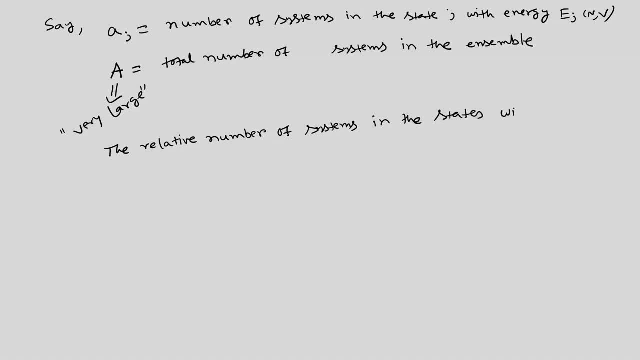 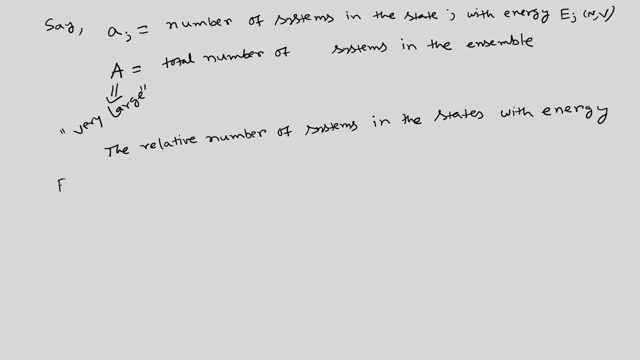 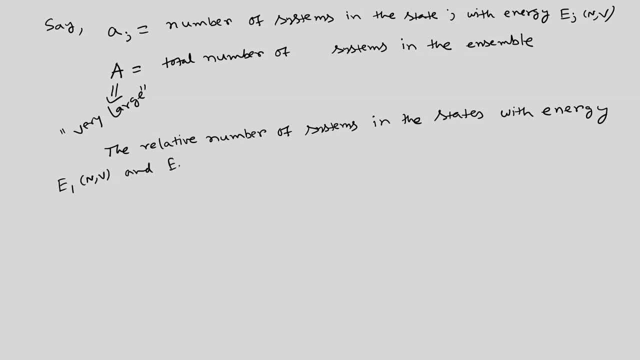 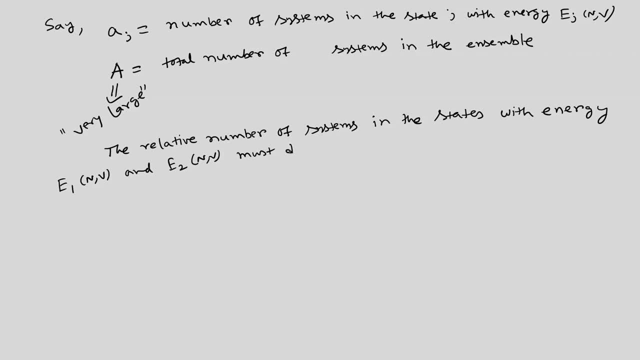 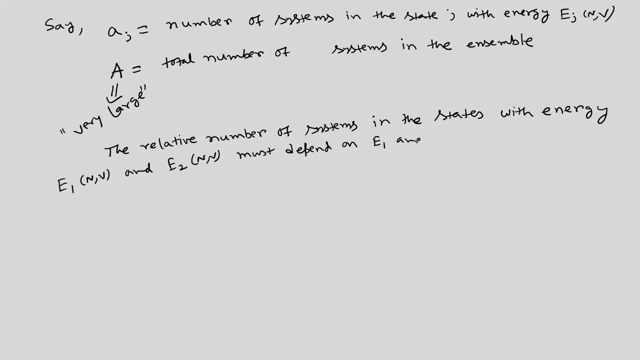 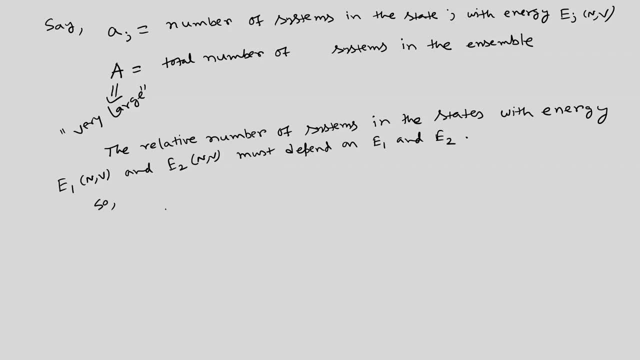 So you can write A2 by A1. is it depends on E1 and E2? okay, okay, So what are? what is E2 and E1? okay, So A2 is the number of states, E2. Okay, Okay. 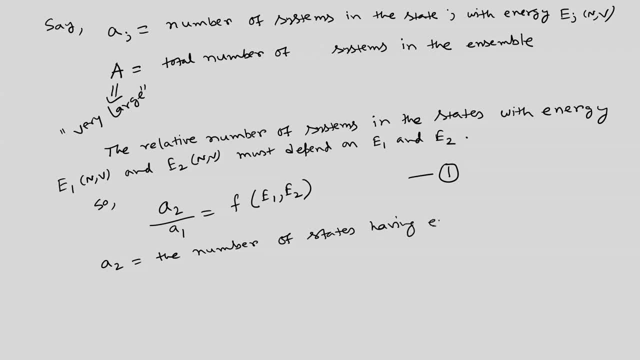 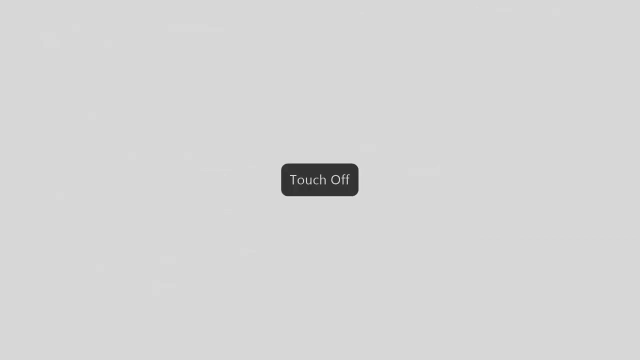 Okay, Okay, Okay, Okay, Okay, having energy E2 and A1 is the number of states having energy E1. fine, okay, Now, since, since energy is a quantity that depends or that must, That must always be referred to a zero energy. 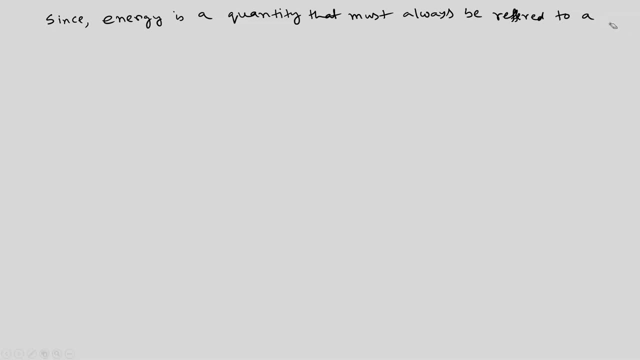 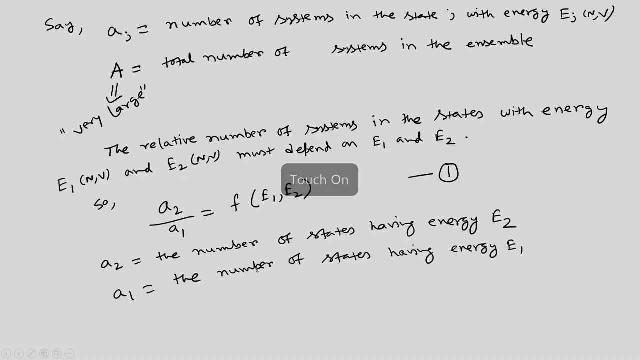 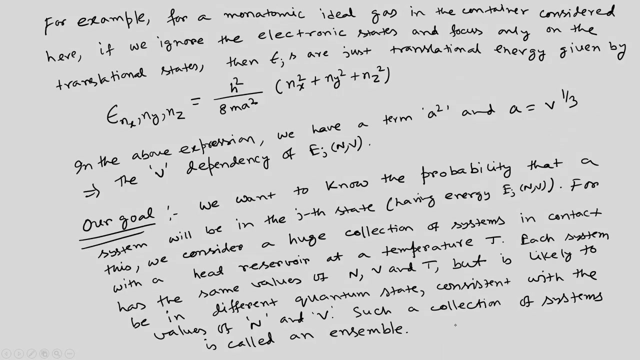 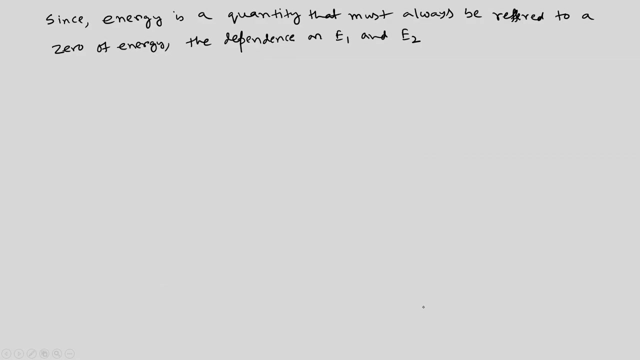 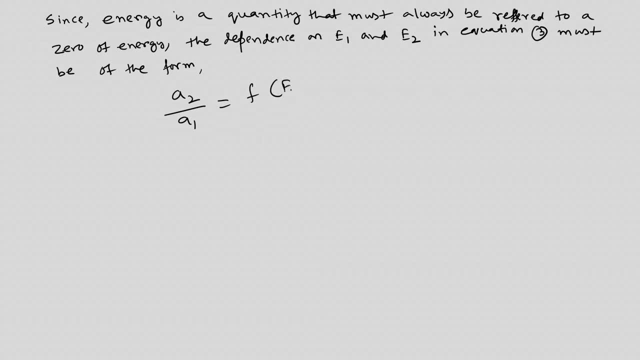 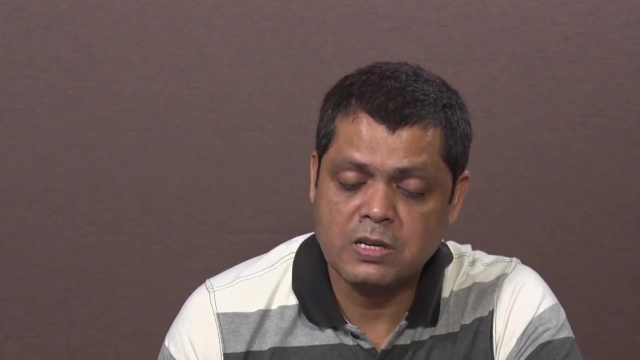 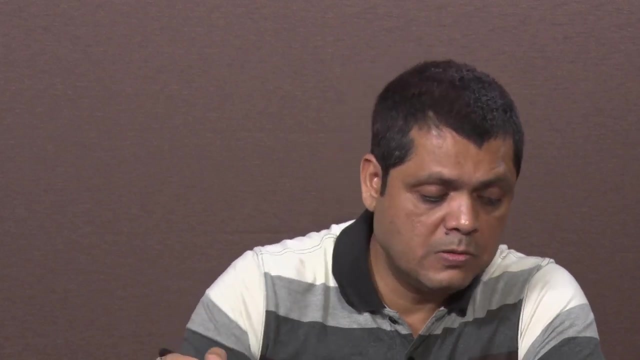 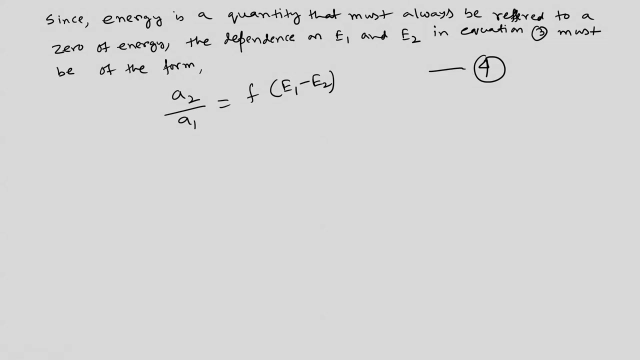 So now this equation four. this equation four is true for any two energy states. Thus we can write that A3 by A2 equals to this function of E2 minus E3 and A3 by A1 function of E1. the difference in E1 and E3, or again A3 by A1, is nothing but A2 by. 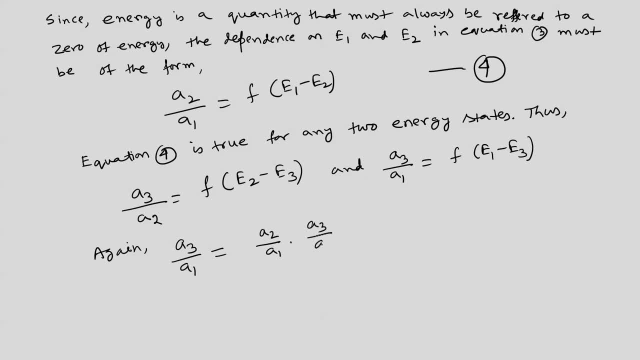 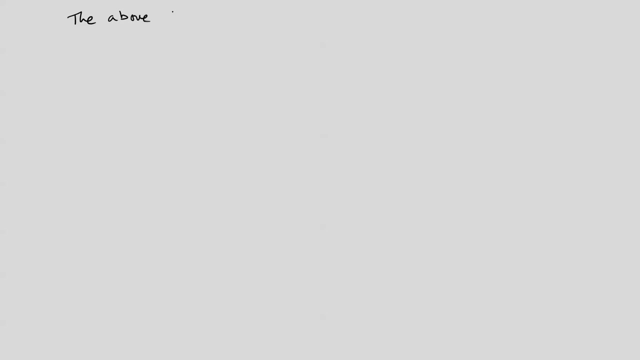 A1 times A3 by A2.. So it says: if E1 minus E3 is right, So suppose this is our equation number 5. okay, This equation 5, So the above equation 5, is very similar to E to the x plus y, is E to the x times E to. 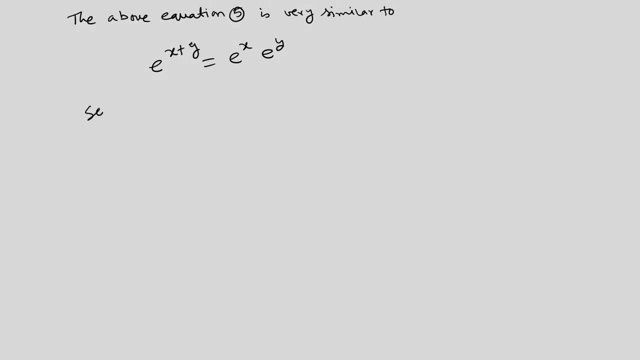 the y. So we can write So A2 by A1.. So A2 by A2 is nothing but E to the beta, E1 minus E2. okay, So this is our equation number 6.. 10.. 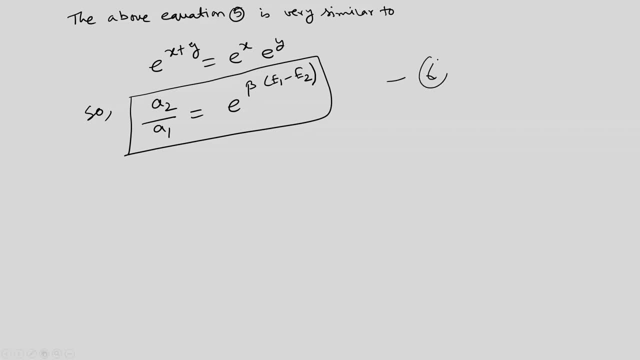 10. This is our equation number 6.. So in general you have: beta is a constant and we will later see that beta is inversely proportional to absolute temperature. Later we will see or we can write: beta is 1, K B T, where K B is the Boltzmann's constant. 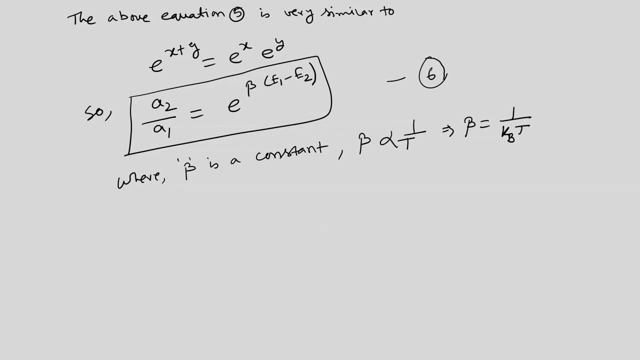 That data. we will prove it. So here beta is a constant for time being 0.. So in general equation 6 can be written as a m by a n is e to the beta e m minus a n. Right? Or you can write a m is sorry, this is a n minus e n minus e m. So in general you can. 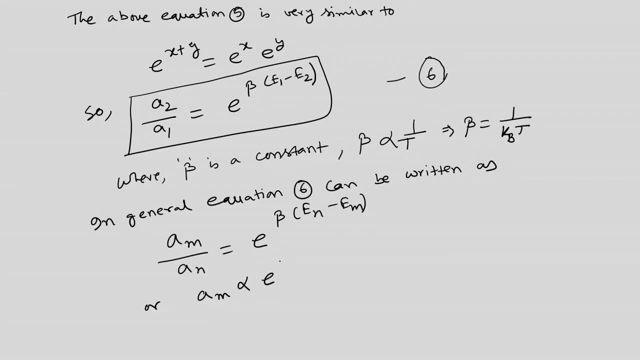 write a m is proportional to e to the minus beta times e m. Or you can write: a m is nothing but c times e to the minus beta a m. Okay, Since a m is a dummy variable, so we can write: a j is nothing but c times e to the minus beta e j. Okay. So for jth state, this is also. 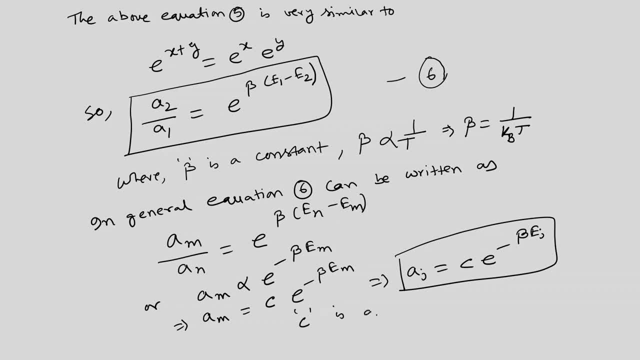 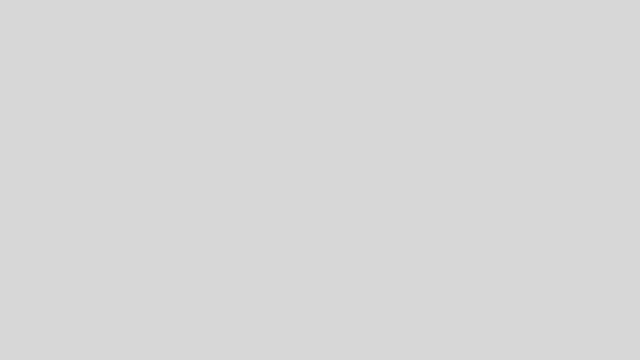 valid where c is a proportionality constant. Right, Okay. So what is the value of c? We will see it, Okay. So what do we get? We get a. j is c times e to the minus beta, e j. Okay, Now, what is the value of c? We will see it. So what is? 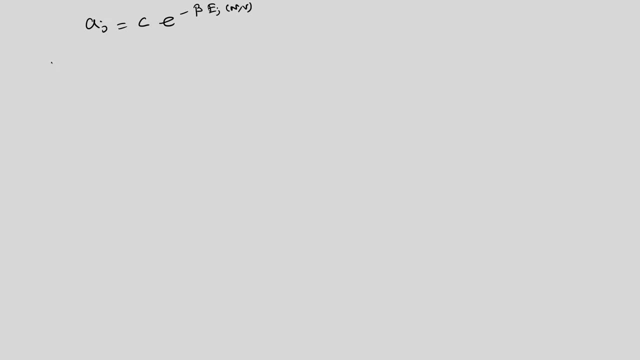 the value of c? We will see it, Okay. So what is the value of c? We will see it. So what is the value of c? We will see it. So what is the value of c? We will see it, Okay Now. 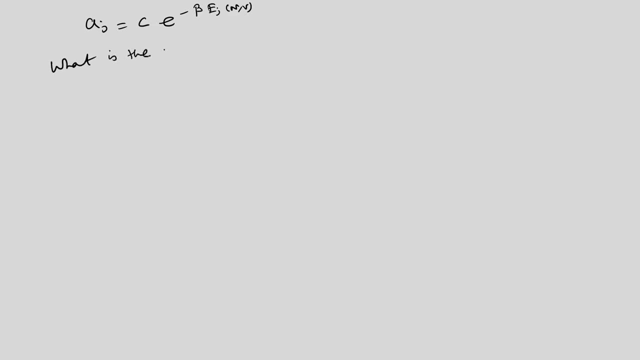 what is the value of c, Of c, the proportionality constant? Okay, So sum over j is a, nothing but a total number of states, Right, And is c times j e to the minus beta j m v. Okay, Or we get c is a by sum over j e to the minus beta j m v. So if you substitute the value 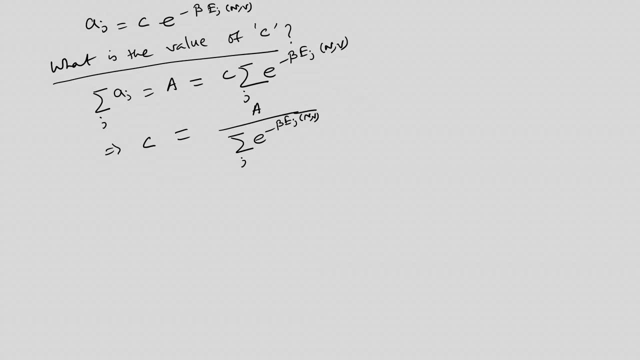 of c in above equation of a j, we get. So we get a j e to the minus beta j m v. Okay, Okay. So that is a e to the minus beta e j by sum over j e to the minus beta e j, Or you can. 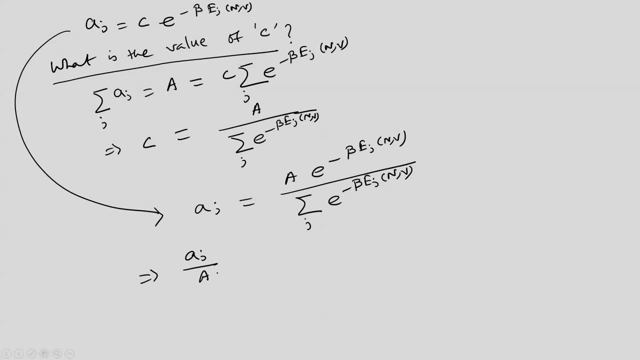 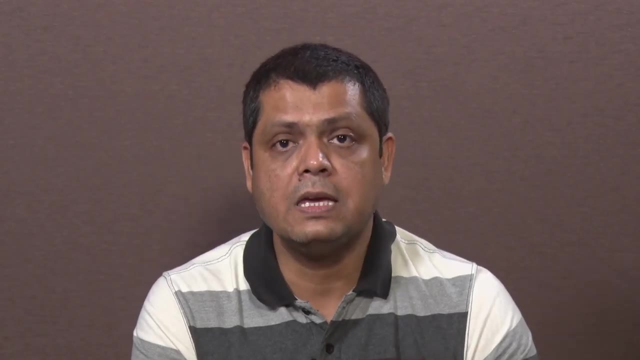 write a j by a. So what is a j by a? You have, we have, Okay, So that is a j. number of states having energy, E, j and capital. a is the total number of steps, Total number of states. So what is a j by a? A j by a is nothing but the probability. 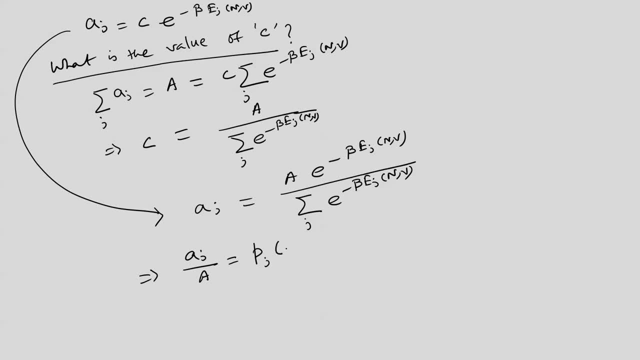 of j, th state having energy E j, So p j. if you say probability, This is probability of e j, Okay, Okay. Okay Okay. state J having energy Ea. So probability depends on Nv beta. we can write e to the. 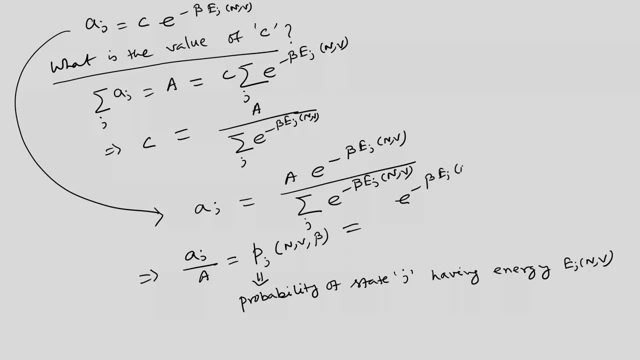 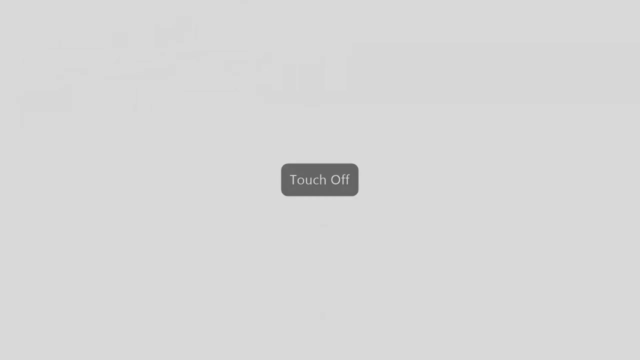 e minus beta ej nv by sum over J: e to the minus beta ej nv, And this J is sum over states. So what we obtain so far, We obtain pj nv: e to the minus e to the minus e to the minus beta ej. 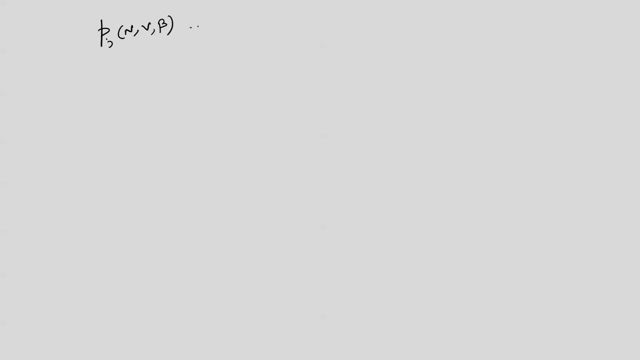 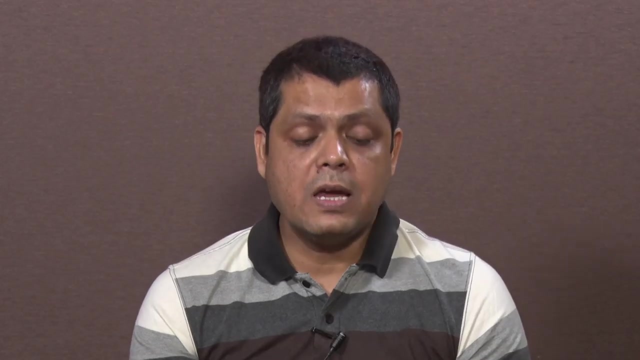 Okay, Okay, Okay, Okay, Okay, Okay, Okay. So pj is function of nv and beta is e to the minus beta ej by sum over j, e to the minus beta ej, nv. So what was our goal? Our goal is to get the probability of state j having. 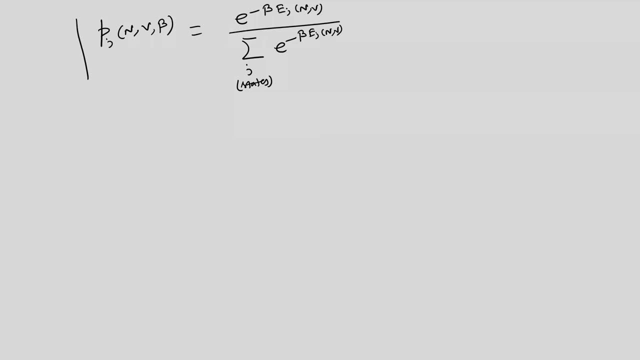 energy, ej. that we arrived at. So this is the expression for that And the denominator we have sum over j, e to the minus beta, ej, nv. So j is sum over states. We define it as q and this q is known as canonical partition function. So our the expression of pj now reduces to: